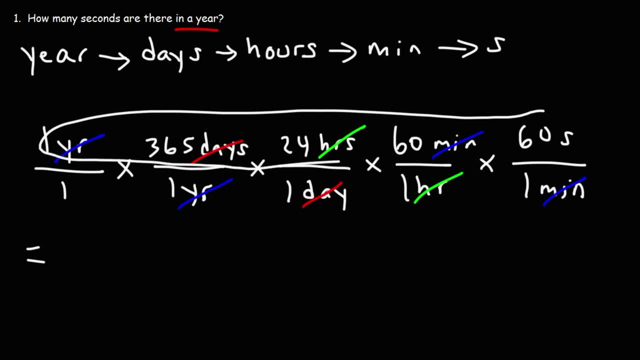 need to multiply by all of the numbers on the numerators of the fractions. So it's going to be 1 times 365 times 24 times 60 times 60. The answer is going to be 31,536,000 seconds. 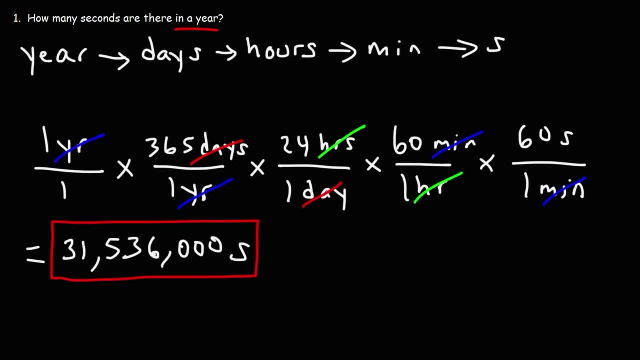 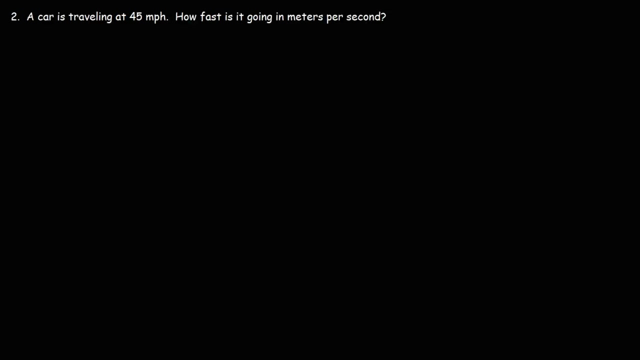 So that's how many seconds there are in a year that's defined as 365 days. Now, if you choose 365.25, your answer will change slightly. It would be 31,557,600 seconds. Let's move on to the next problem. A car is traveling. 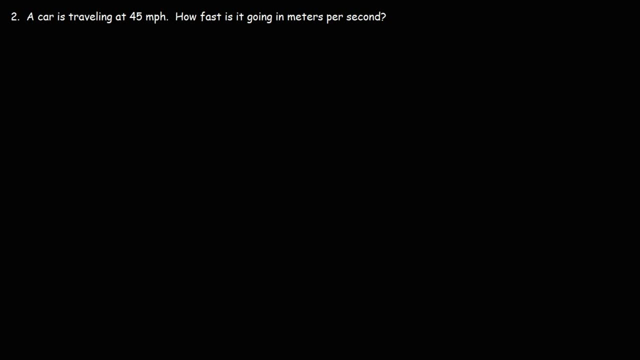 at 45 miles per hour, How fast is it going in meters per second? So how can we convert from miles per hour to meters per second? So this is a two-part problem. First, we need to convert the units of length, miles, to meters. 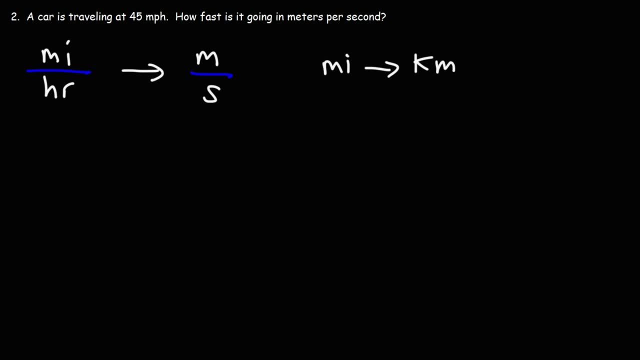 What we could do is convert miles to kilometers and then kilometers to meters. Next, we need to convert the units of time from hours to seconds, which we already know how to do. We can convert from hours to minutes and then minutes to seconds. Now it's helpful to write the conversion factors that you're going to use. One mile is equal. 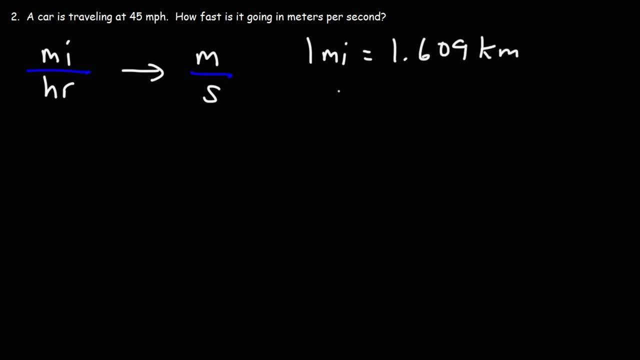 to 1.609 kilometers per hour. Think of the word kilo. A kilo is 1,000, so one kilometer is 1,000 meters, And we know that one hour is equal to 60 minutes and one minute is equal to 60 seconds. So those are. 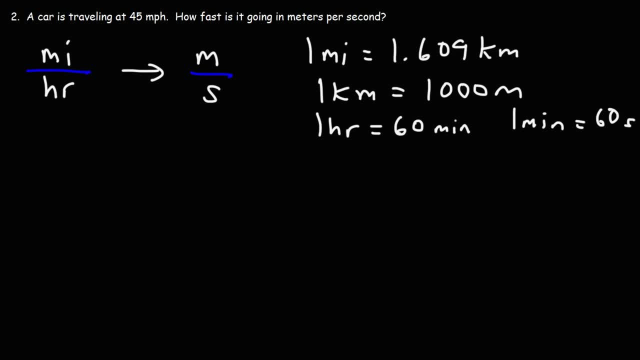 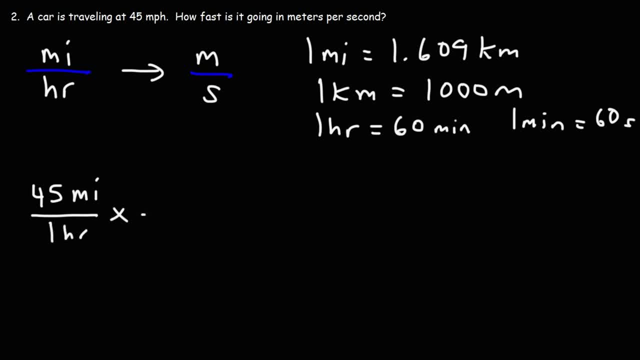 So we have 45 miles per hour. So we have 45 miles per hour. So we have 45 miles per hour. And let's convert miles to kilometers. So we have miles on top. we want to put the same unit on the bottom. So here's our conversion factor. I'm going to put this part on the 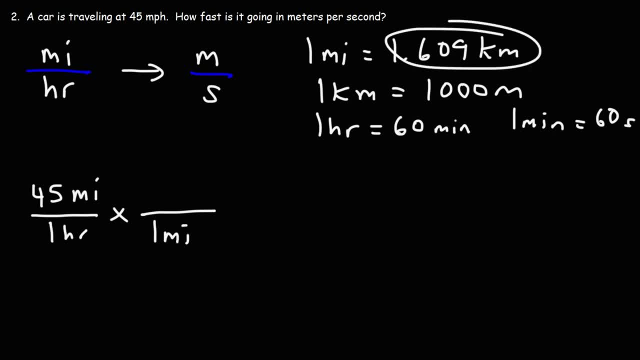 bottom of the second fraction and then the other part on the top of the second fraction. So the unit's miles will cancel. Now let's use our next conversion factor to convert from kilometers to kilometers to meters. So since we have kilometers on top in the second fraction, I'm going to put 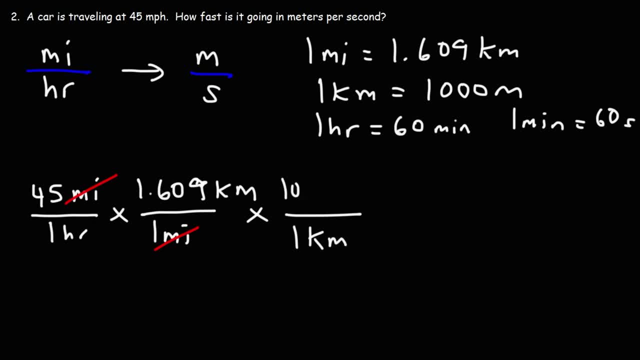 kilometers on the bottom of the third fraction, And then the other side of the equation is going to go on top. So now we can cross out kilometers, So we have our desired unit meters, so we can leave that alone. Now let's focus on units of time. Let's convert hours to seconds, But first 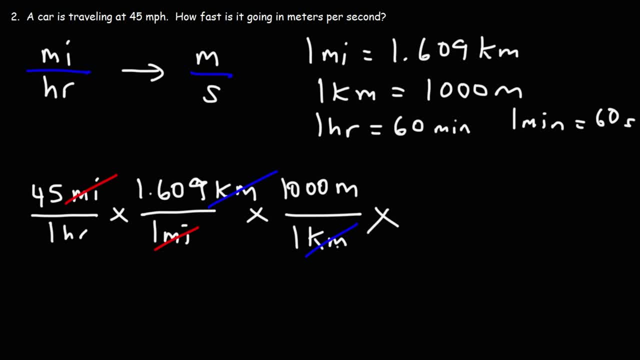 we'll convert hours to minutes, So let's use this conversion factor. Notice, we have hours on the bottom, so we need to put it on top of the fourth fraction. So we're going to put this here. The other part of the conversion factor is going to go on the bottom. 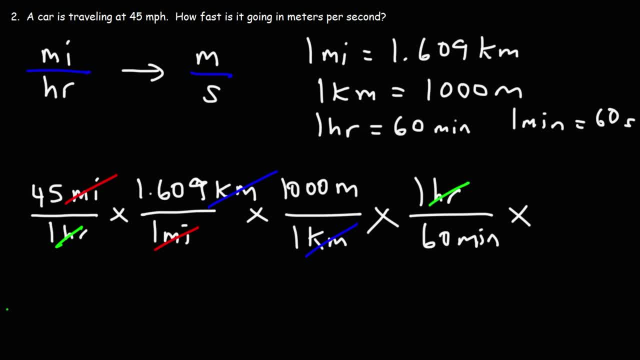 So now we can cross out hours. Finally, we can use the last conversion factor to go from minutes to seconds, And now we can cross out the unit minutes. So we're left with meters on top and seconds on the bottom, So we have the speed in meters per second. 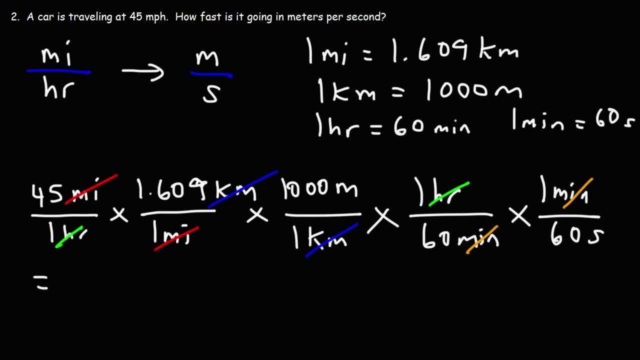 So now we need to do the math. Everywhere you see a 1, you can ignore. We're going to multiply by the numbers on top and then divide by the numbers on the bottom. Let's begin. It's going to be 45 times 1.609 times 1000, divided by 60, and then divide that result by 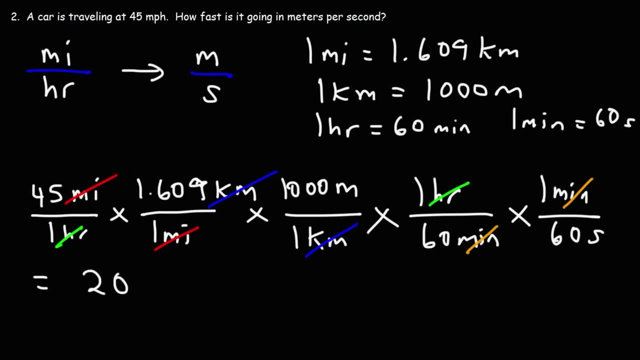 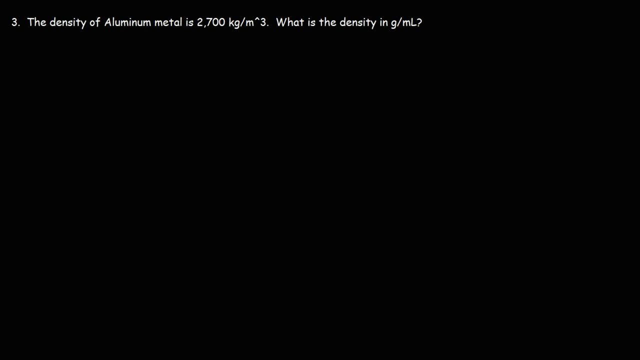 60. So you should get 20.1 meters per second. So that's how you can convert from miles per hour to meters per second. Now let's move on to number three. The density of aluminum metal is 2700 kilograms per cubic meter. 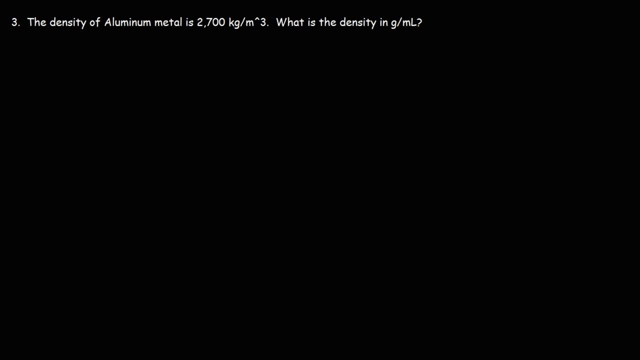 What is the density in grams per milliliter? Go ahead and try that one. So we're given the density in kilograms per cubic meter And we want to convert it to the density in grams per milliliter. So we need to convert the mass from kilograms to grams. We could do that in a single step. 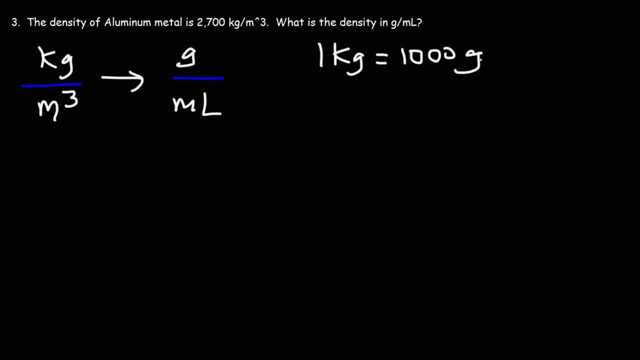 One kilogram is 1000 grams, And then we need to convert the volume portion of density from cubic meters to milliliters. So what we can do is convert cubic meters to cubic centimeters. By the way, one meter is 100 centimeters. 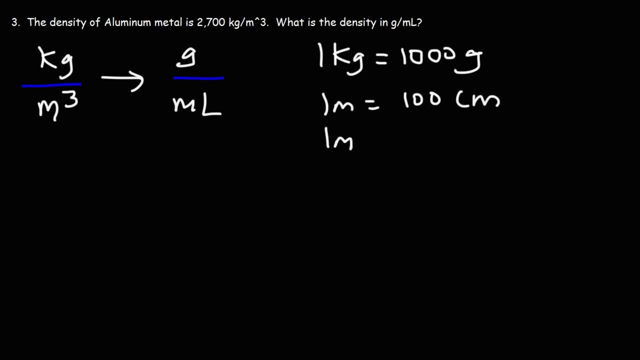 And then we can convert cubic centimeters to milliliters. One milliliter is equivalent to one cubic centimeter. So let's begin. We're given 2700 kilograms per cubic meter. That's the density of aluminum metal. We could use this one to go from kilograms to grams. 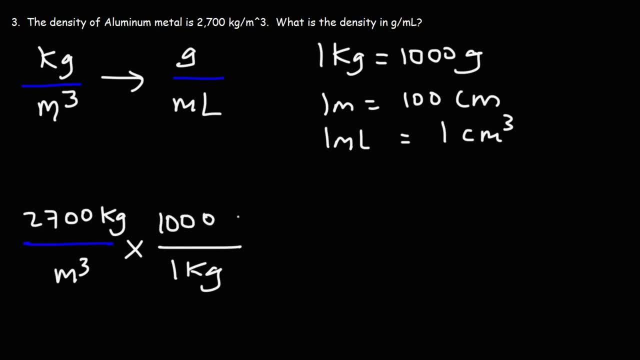 So one kilogram is equivalent to 1000 grams. So now we can convert this to grams per cubic meter. So now we can cross out the unit kilograms. Now let's use the next one. Let's go from meters to centimeters. 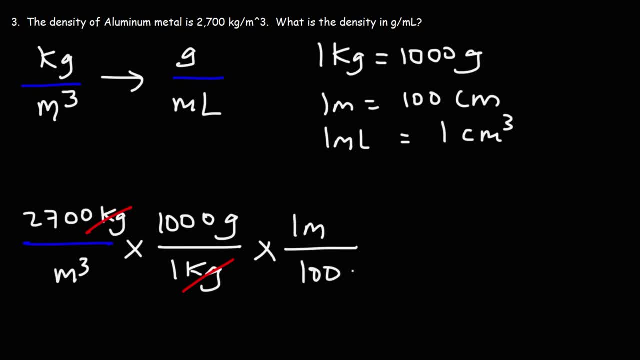 We know that 1 meter is equal to 100 centimeters. Since we have meters on the bottom, I decided to put meters on top in a third fraction. But now this is the part you need to pay special attention to. Notice that we don't just have meters. 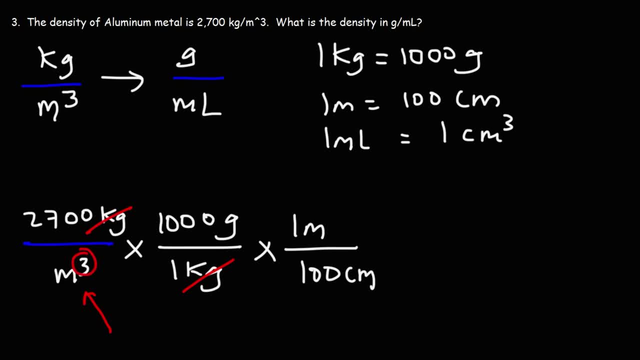 We have cubic meters. That's a meter times a meter times a meter. What we need to do is raise this to the third power, So this becomes cubic meters If we raise this to the third power. 1 meter raised to the third power, that's 1 meter times 1 meter times 1 meter. 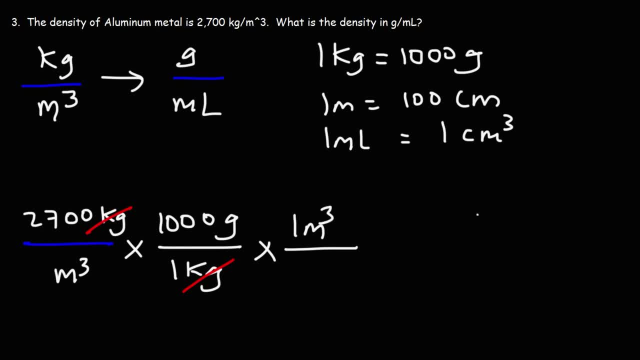 That becomes 1 meter cubed, Now 100 centimeters. If we raise this to the third power, that's 100 centimeters times 100 centimeters times 100 centimeters. So that is 1 million cubic centimeters. 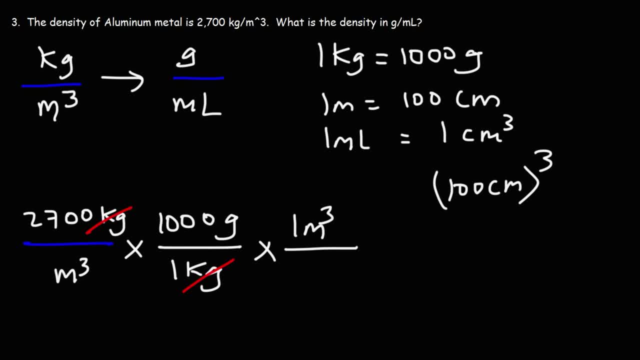 Or you can write it as: 1 times 10 to the 6th, 1 times 10 to the 6th. So basically what you do is you can take the cube of this equation and you get: 1 cubic meter is equal to. 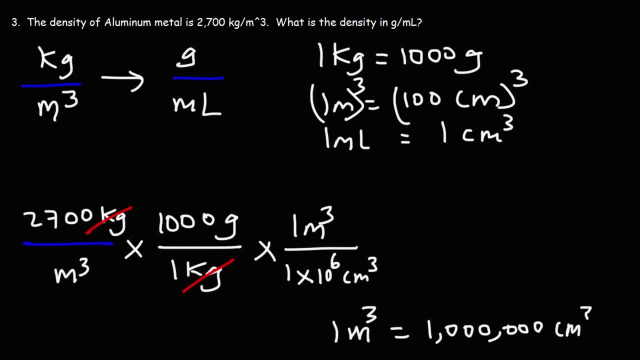 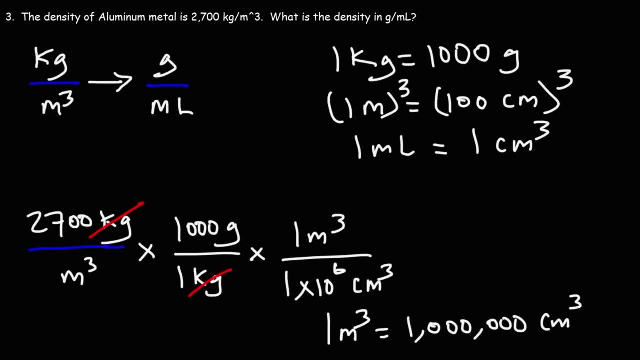 a million cubic centimeters. So now we can cross out the unit cubic meters. If you're wondering why the screen looks a little different, I had to do some video editing. Now let's finish this problem. So right now we can cross out the unit cubic meters. 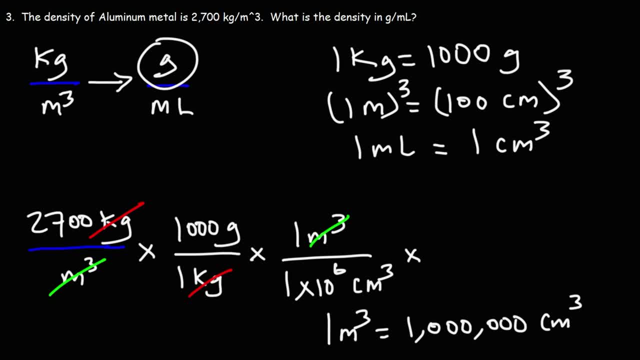 We have grams on top, but we need to get milliliters on the bottom, So we could use our final conversion factor. 1 cubic centimeter is equal to 1 milliliter, So now we could cancel the unit cubic centimeters. 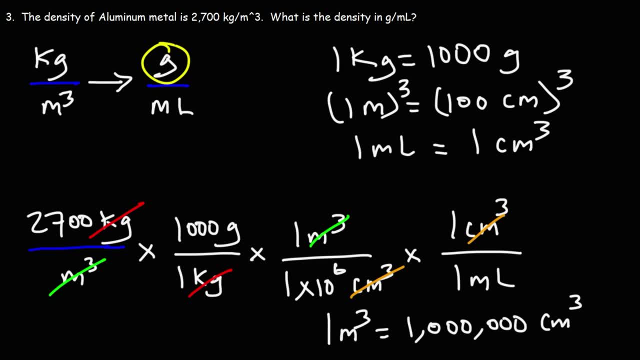 So what we have is the unit grams on top and the unit milliliters on the bottom. So now we just got to do the math. So we're going to multiply 2700 by 1000, and take that result. 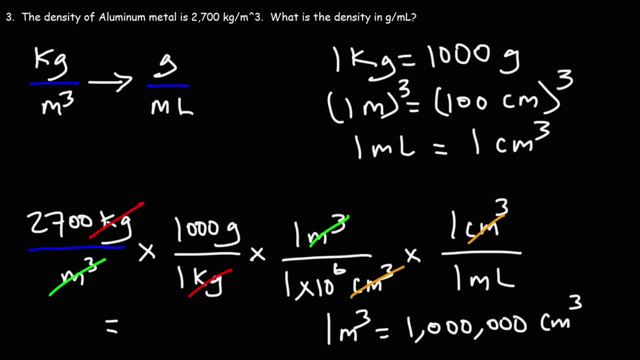 divide it by a million, or 1 times 10 to the 6th, The final answer is going to be 2.7 grams per milliliter. Any time you need to convert from kilograms per cubic meter to grams per milliliter. 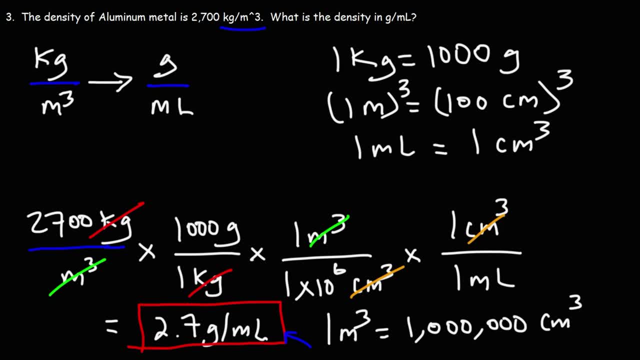 simply divide by 1000.. Because in physics the density of objects are typically reported in kilograms per cubic meter, But in chemistry you'll find that the density is usually reported in grams per milliliter. So this is a common conversion that. 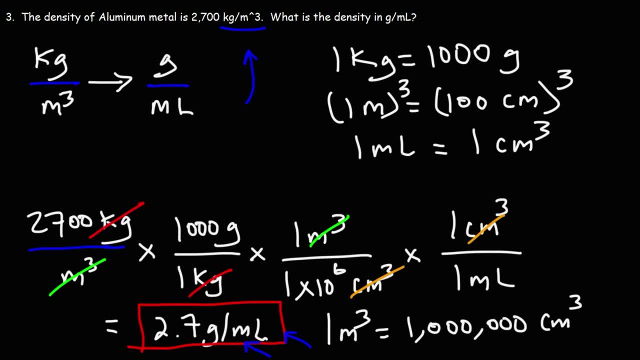 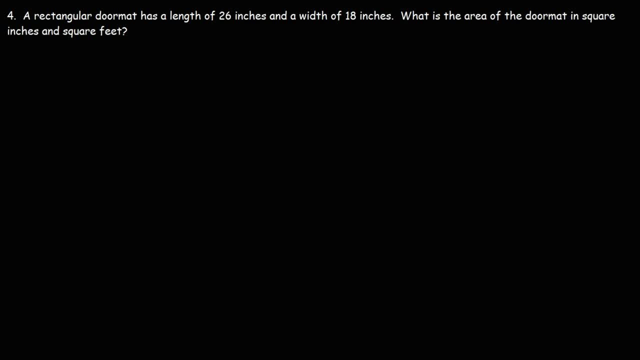 you may encounter when going between physics and chemistry. Number 4. A rectangular doormat has a length of 26 inches and a width of 18 inches. What is the area of the doormat in square inches and square feet? 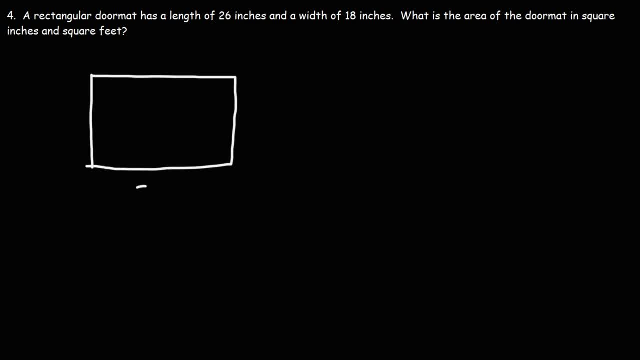 So let's draw a picture. Let's say this is the doormat. The length is 26 inches, the width is 18 inches. To calculate the area, the area of a rectangle is the length times the width. It's L times W. 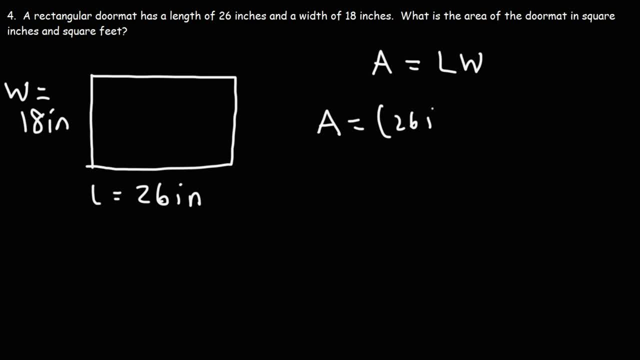 So in this example we need to multiply 26 inches by 18 inches, This is going to be 468.. Now we're multiplying inches to the first power, times inches to the first power. So when you multiply by a common base, you need to add the exponents. 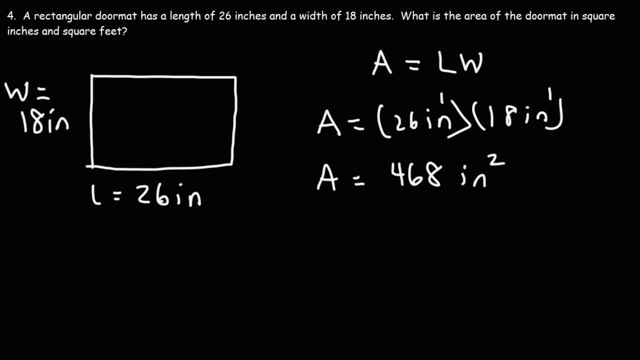 1 plus 1 is 2.. So we get the area in square inches. So we get the area in square inches. So that's the answer to the first part of the question. Now we need to get the area in square feet. 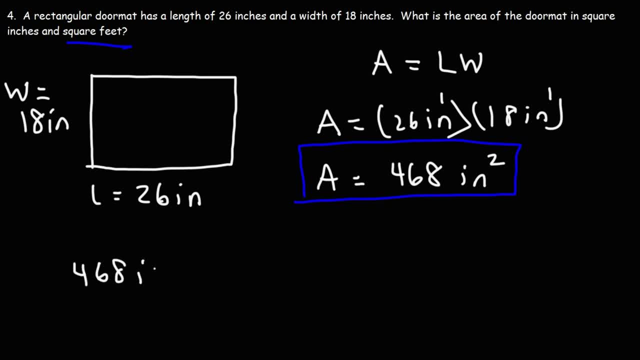 So we're going to convert it from square inches to square feet. So how many inches in a foot? We know that there's 12 inches in one foot. So we have inches on the top left, but we're going to put it on the bottom right. 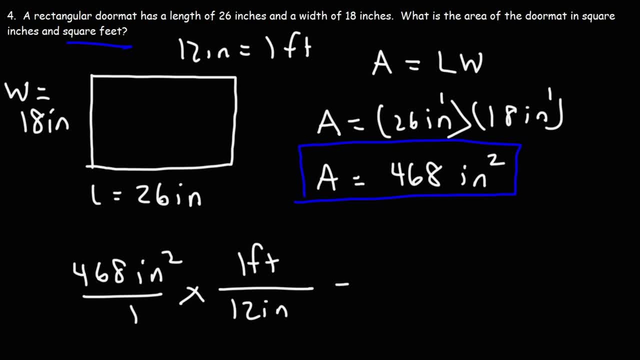 Now notice that it's inches squared, So we need to square this conversion factor so we can get square feet. So the answer is going to be 468 divided by 12 squared. 12 squared is 144.. So you should get 3.25 square feet. 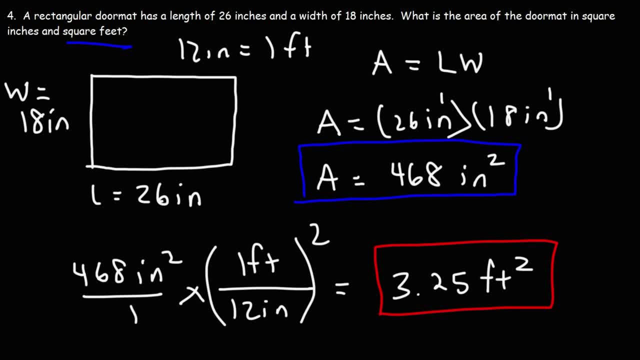 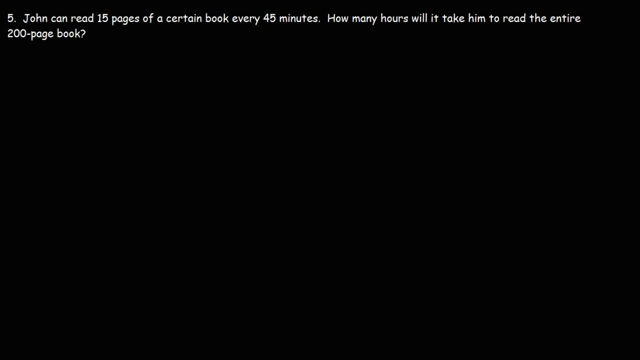 as your final answer. So that's how you can convert from square inches to square feet. So that's how you can convert from square inches to square feet. Number five: John can read 15 pages of a certain book every 45 minutes. 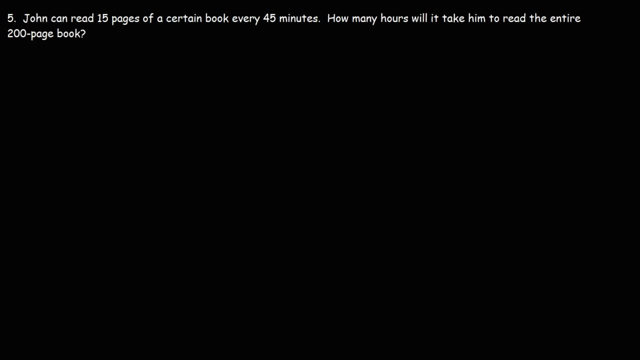 How many hours will it take him to read the entire 200-page book? to read the entire 200-page book? So think about what we're given. So think about what we're given. We're given 200 pages And from that. 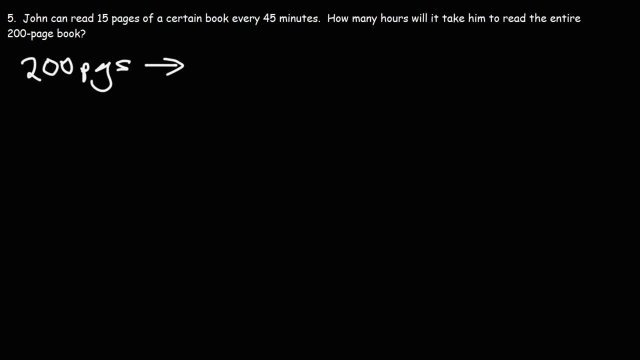 And from that we need to find out hours, How many hours it will take him to read 200 pages. So we're converting pages to hours. How can we do this? What conversion factors do we have to go from pages to hours?